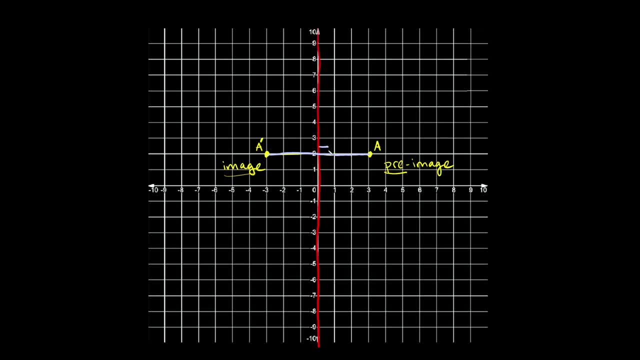 to the other point, it has to create a perpendicular angle or 90 degree angle with the line of reflection. Okay, So, for example, if I drew a line, a point, right here and called this A prime, well, is this really a reflection of this original point? No, it's not Okay. 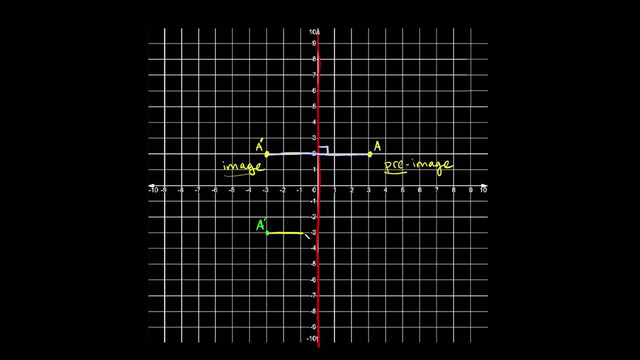 Because, as you can see, this point right here is also three spaces away from the line of reflection, Right? But if I draw a straight line from my original point to this other copied point, it doesn't make a 90 degree angle here, Right? This is more like a maybe 60 degree angle. 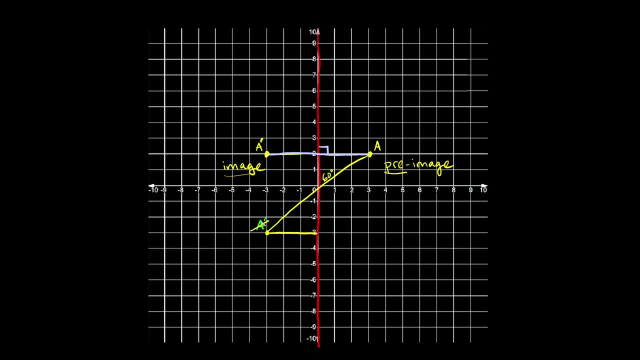 or something, Right? So that would mean that this point right here is not a reflection of this point right here. Okay, Remember, the two points have to create this perpendicular angle. Okay, So we reflected this point across the Y axis, Now let's reflect it across the. 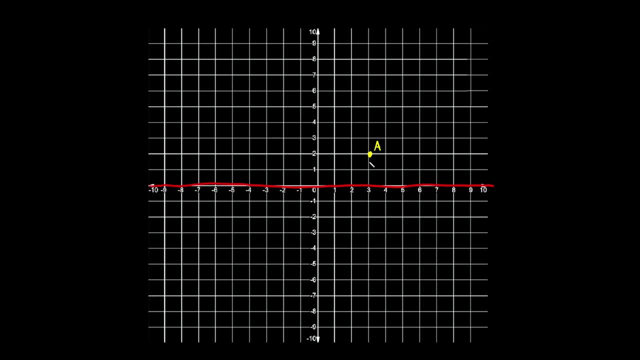 Y axis, right here. Okay. So again, if I want to reflect this point across this line right here, well, point A, right here, is one, two spaces away from the line Right. So then our copied point, or reflected point would be one, two spaces away also. Okay. So this: 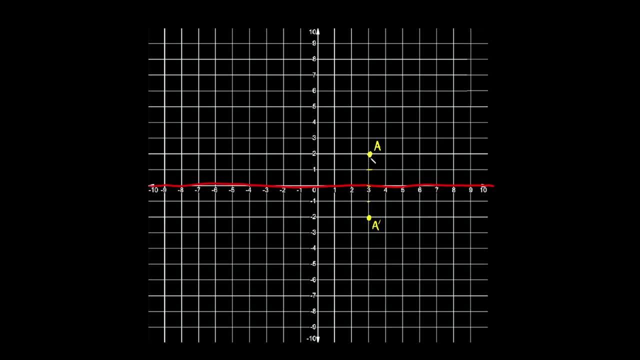 would be A prime right there. And again, you can see that if I draw a straight line from one point to the other, it would make a 90 degree angle with the line of reflection Right. Okay, We're going to switch it up a little bit this time. So now this is point. 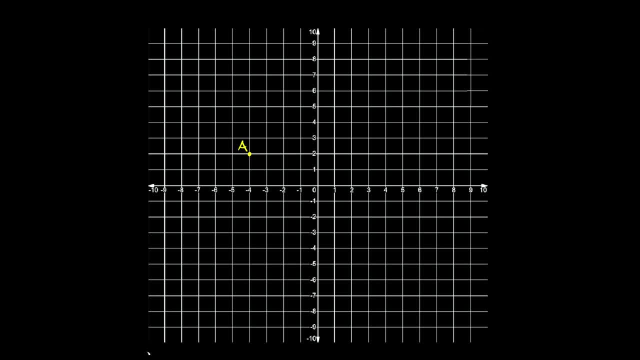 A right here, And let's draw our line of reflection at an angle, specifically at: Y is equal to X, Okay, And Y is equal to X is basically just a straight line like that: Right, Y is equal to X has a slope, positive one that runs through the origin, right here, Okay. So this is point A right here. Now. 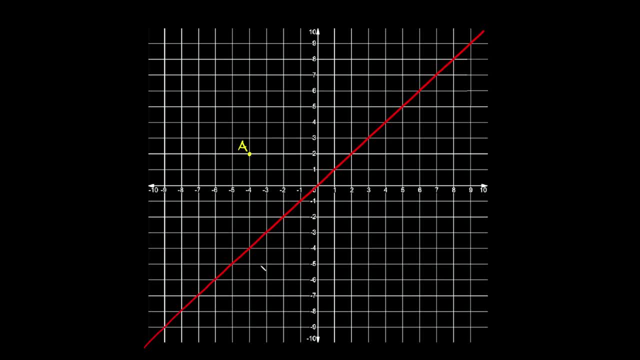 how would we reflect point A across this line of reflection? Well, there's basically a few different ways we can do that. So, first of all, we can count spaces again, but this time we're going to count diagonal spaces, Okay, So we'd. 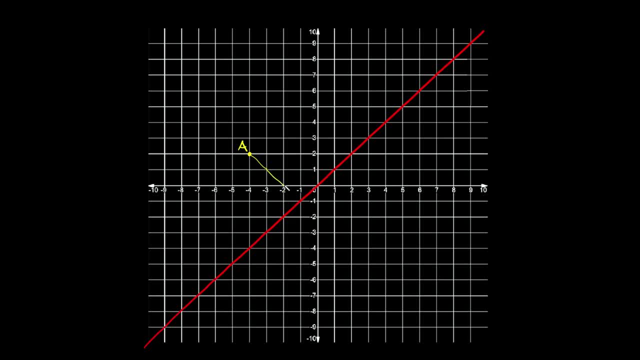 basically say we get one, two, three diagonal spaces, right. So then point A on this side would be one, two, three spaces away, like that. Okay, So then that means this is a prime right there, Okay, And as you can see, this straight line between the two points makes a perpendicular. 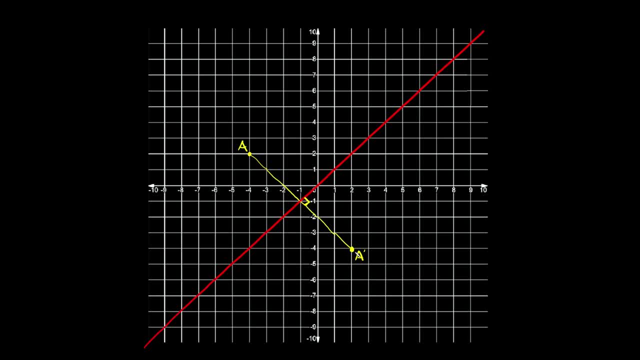 angle with the line of reflection. right Now, another way that we could count the spaces is basically just start at your original instead of 3, 4,, 5,, 10,, 8 необходимо. and if you're doing that with a two- 왜 Esp tires right there, Okay. And as you can see, this straight line between the two points makes a perpendicular angle with the line of reflection. right now, another way that we could count the spaces is: 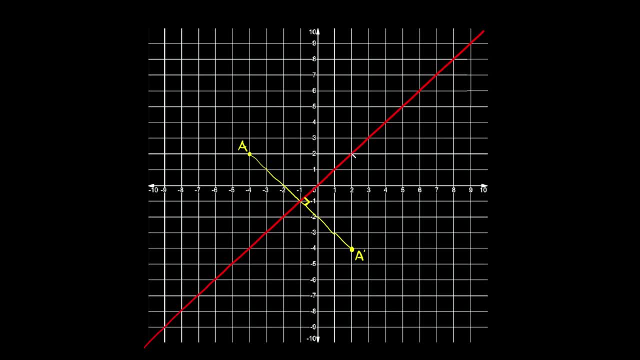 start at your original point and then just go in a straight line until you hit the line of reflection. okay, you can either go sideways or you could go down. in this case, it doesn't matter, works either way. so here we would go one, two, three, four, five, six spaces. right? so then from here we would go down six spaces. 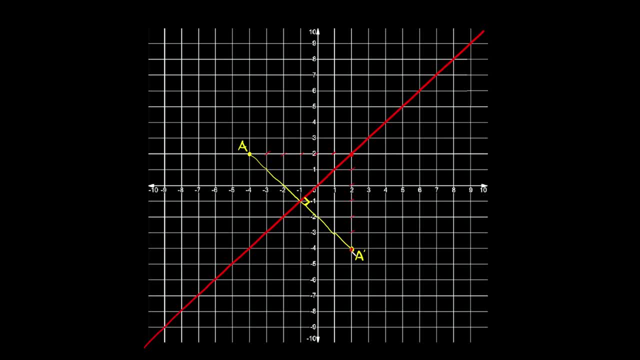 one, two, three, four, five, six, and then we land at a prime again. right, okay. now what if I wanted to reflect a line like this across the line of reflection? well, it's still the same steps, okay. the only difference here is we're basically going to reflect two points. okay, because we have point A and point B. okay, so first, 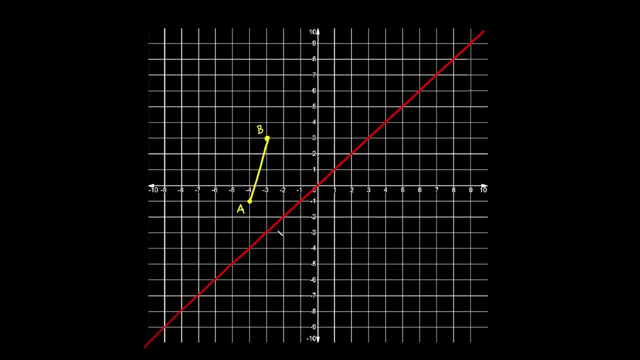 of all, if we wanted to reflect point A right here again, how far is it from this line right here? well, it's one diagonal space, one and a half right. so it's one and a half spaces away. so then we go half, one and a half right. so then this: 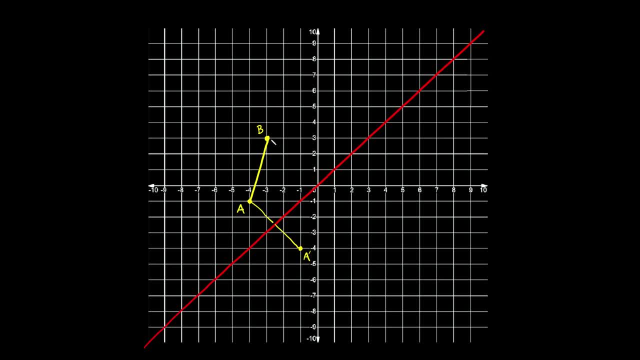 point right here would be a prime and then B- same thing. how far is it from the line of reflection? well, it's one, two, three spaces away, right? so then we'd go one, two, three spaces away to right there. so then this point right here would be B, prime, okay. and then you would. 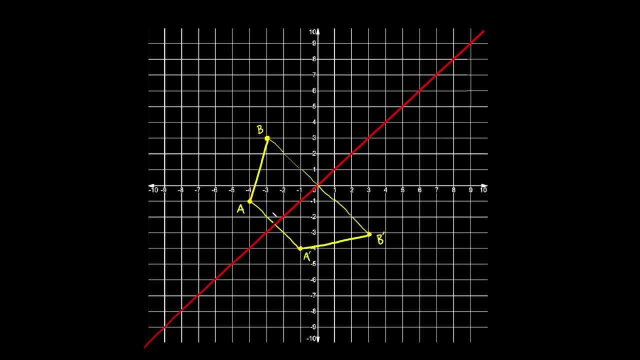 just draw a straight line from a to B and again the straight lines from a to a prime. this makes a perpendicular angle. and from B to B prime. this also makes a perpendicular angle. all right now. one more kind of example that trips people up sometimes is: let's say, we wanted to. 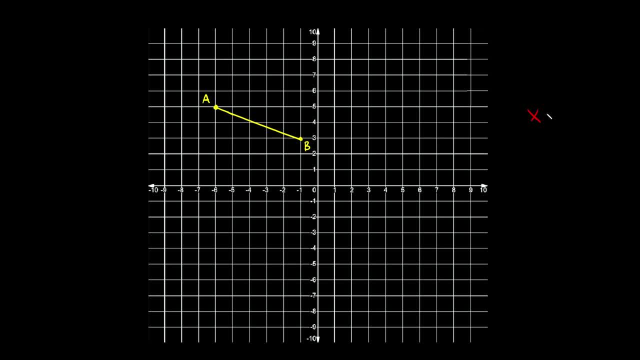 reflect this point across the line. let's say: X is equal to negative 3. okay, well, this is the x-axis. negative 3 is right there, right? so X is equal to negative 3. is this line right here? right? X is equal to negative 3. now, as you can see this, 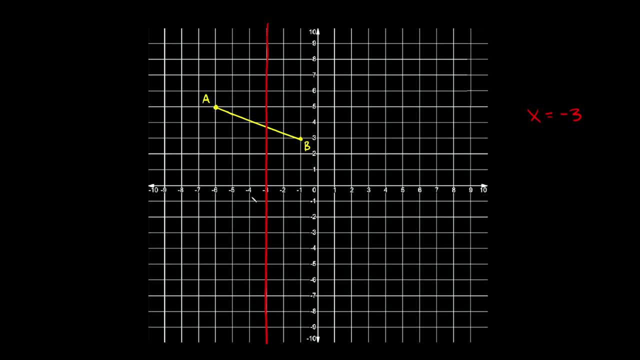 line right here runs through the line of reflection, right. so that's kind of weird, but the same exact rules still apply, okay. so, starting with point a, if I wanted to reflect it across this line right here, well, again, it's 1, 2, 3 spaces. 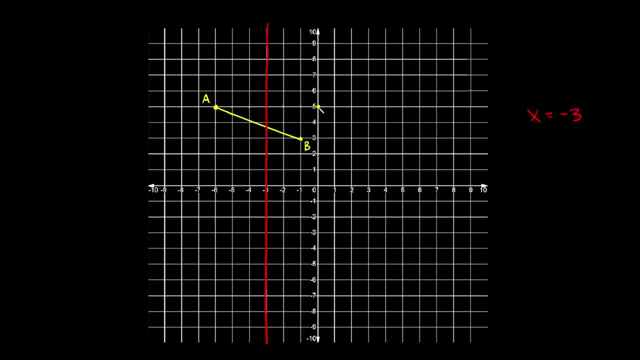 away, right. so then it'd be 1, 2, 3 spaces away in this direction, right here, right. so this would be a prime and then B. right here is 1, 2 spaces away from this line. so then B prime would be 1, 2 spaces away, right there, okay. 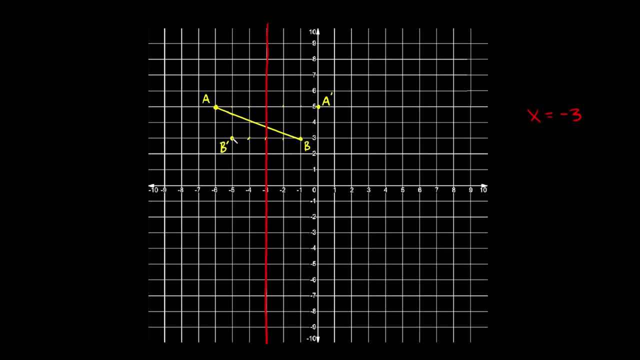 B prime, okay. And then again you would just draw a straight line, right, because we are reflecting the line. So then, from A to B, it's right there. Okay. and as you can see again, if I drew a straight line from A to A, prime, right here. 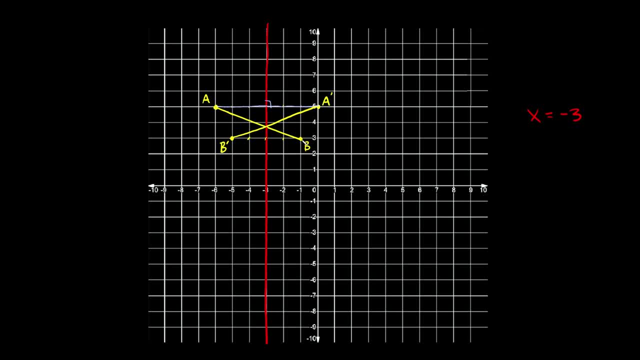 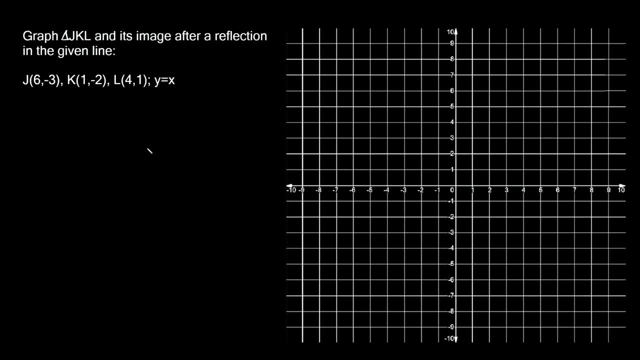 it creates a perpendicular angle right. And if I drew a straight line from B to B prime, it again creates a perpendicular angle. All right, so now let's just run through a couple more examples where we've got to set up the problem a little bit. 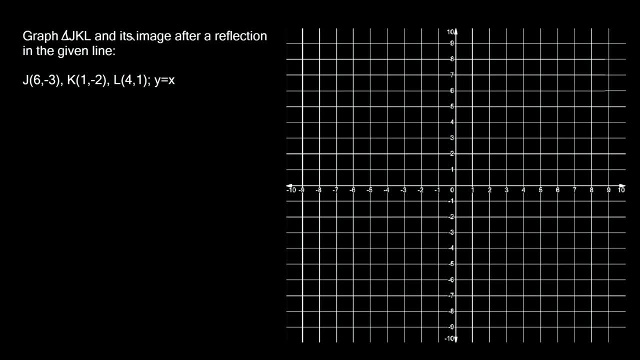 All right. so this one says: graph triangle JKL and its image, or in other words and its copy, after a reflection in the given line. Okay, so it gives us these points to plot. right, to plot triangle JKL. 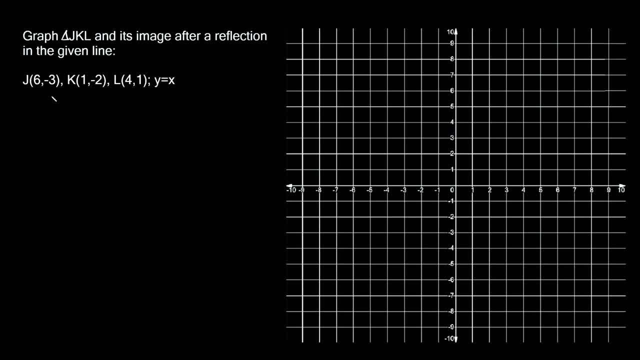 and then we need to reflect it across this line: Y is equal to X. Okay, so, first of all, J right here is at 6, negative 3, right, 6, negative 3.. So that's, J K is at 1, negative 2, 1, negative 2, right. 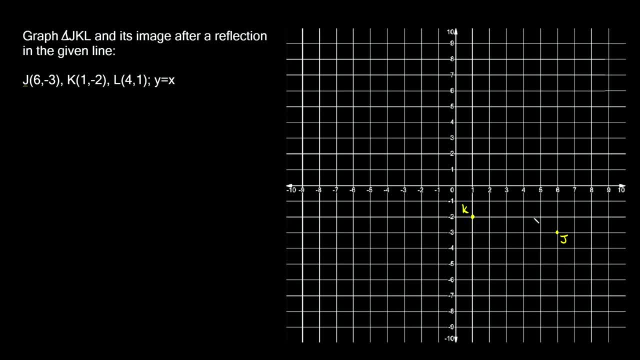 So that's K, Okay, and L is at 4, 1.. So 4, 1 is right there for L, Okay. so this is JKL, Okay. so then let's draw a straight line right there, Boom. 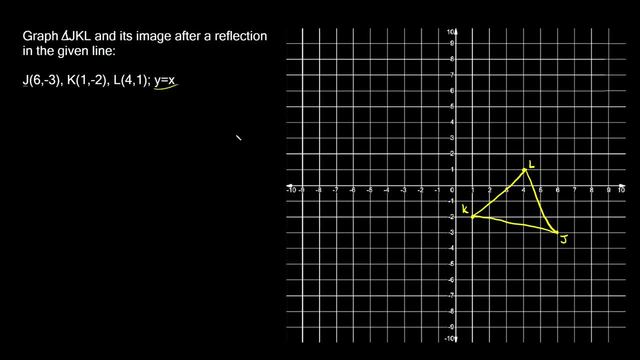 Okay, now we're going to reflect it across. this line, right, Y is equal to X. Now again, Y is equal to X is just that straight 45 degree angle that runs through the center, through the origin, right there. Okay, so that would be this line, right here. 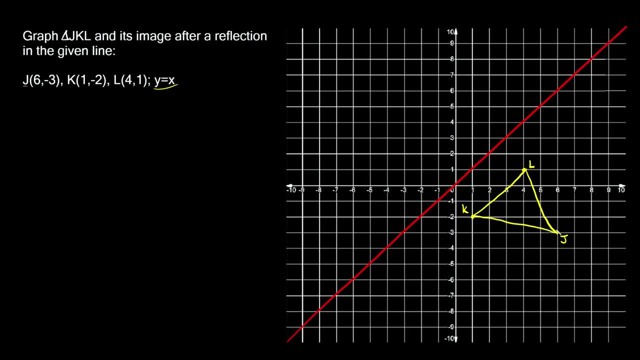 Boom, Nice, Okay. so now let's reflect this triangle and let's just start right here with point J. So how far is point J from the line of reflection? Well, it's 1,, 2,, 3,, 4, and a half right. 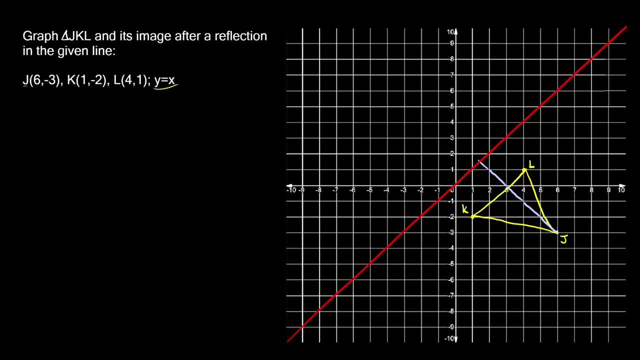 So 4 and a half spaces away. So in this direction we're going to go 4 and a half, So we're going to go 1, or- sorry, this is a half- and then we're going to go 1 and a. 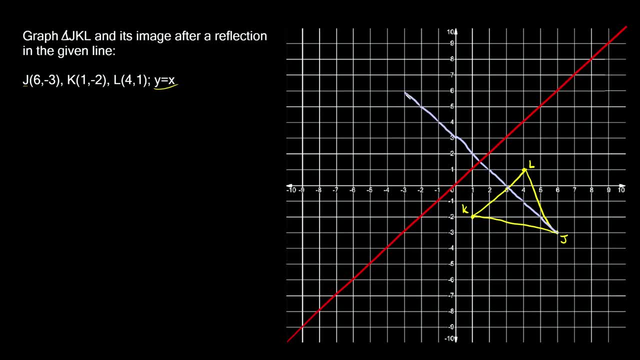 half, 2 and a half, 3 and a half, 4 and a half, right. So then, this point right here, This point right here is J, prime. And then doing the same thing with these two other points: K, right here is 1, and then 1 and a half spaces away, right. 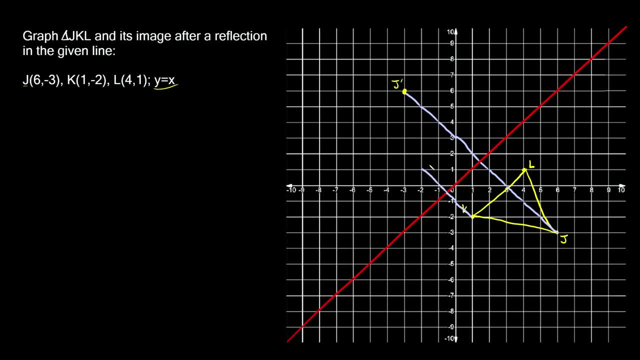 So then, in this direction, we're going to go a half and then 1 and a half, right. So then this is K prime And then L same thing. This is 1,, 1 and a half spaces away. So then we're going to go a half, 1 and a half spaces away, right? 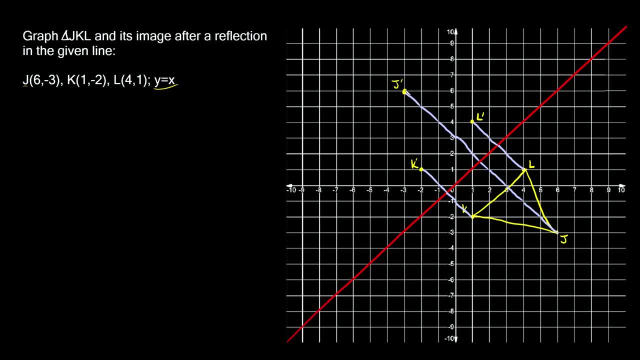 So then this right here would be L prime, And then I plotted all my points. So the last thing we have to do here is just connect our dots to create our triangle. All right, last one. So this one says: graph the polygon and its image or copy after a reflection in the given. 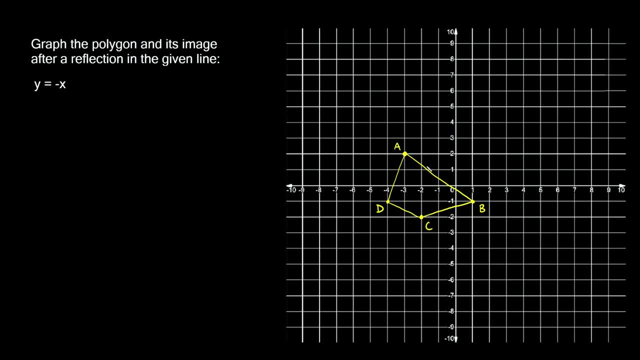 line, And the line it's giving us is: Y is equal to negative X, right? So this is the polygon we're going to graph or reflect across: Y is equal to negative X, right? So remember the last problem we used: Y is equal to X, right? 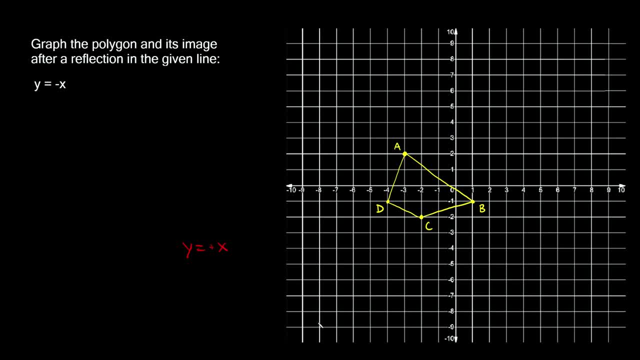 So Y is equal to X, Or in other words, Y is equal to positive X. It gives us a positive slope And that means Y is equal to negative. X would be a negative slope, right? So this would be: Y is equal to negative X. 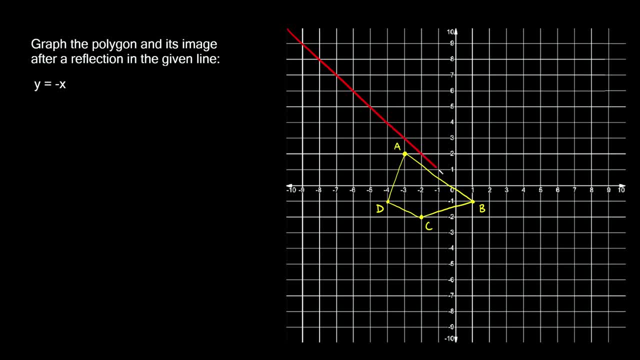 So let's clean this line work up. So this is: Y is equal to negative X, right? So, as you can see, it has a slope of negative 1, right, Y is equal to X has a slope of positive 1.. 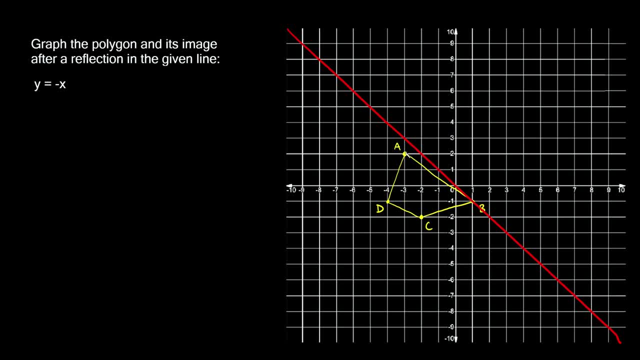 This is negative 1.. All right, now let's start with point A. right here? So point A is half a space away from the line of reflection. right, So A prime is going to also be half a space away from the line of reflection. 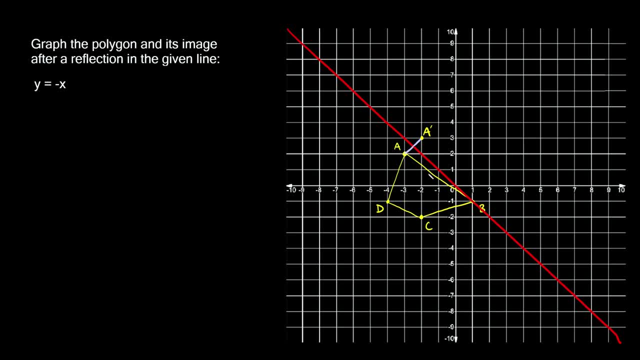 Okay, so this is A prime right there. Okay, now point B. over here. Point B, as you can see, is on the line of reflection. okay, So point B is zero spaces away from the line of reflection. So point B, prime, is also going to be zero spaces away from the line of reflection.